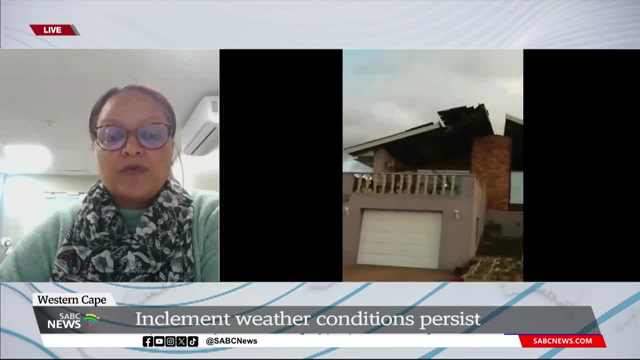 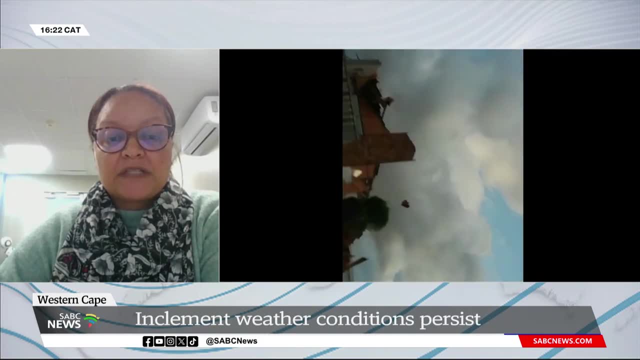 that have been uprooted since Saturday. We've also received some flooding reports from Leonsdale Epping area and Kailitsa, where 12 structures has been flooded. in Emple Wainy Village and also in Monwa BC. We're approximately 4,000 hectares of land. in Monwa BC, We're approximately 4,000 hectares. 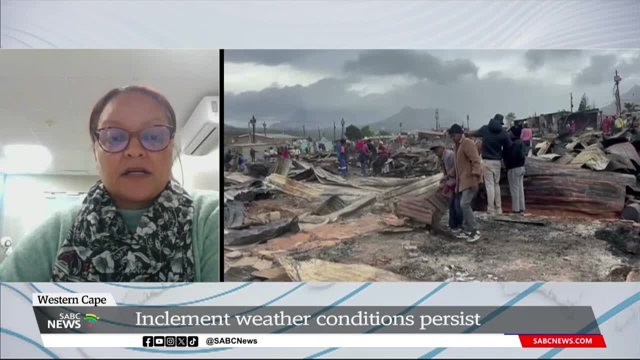 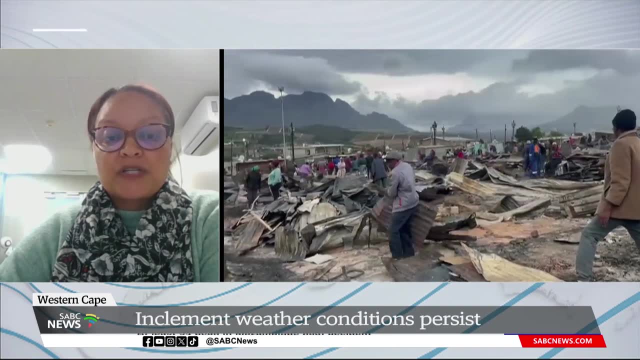 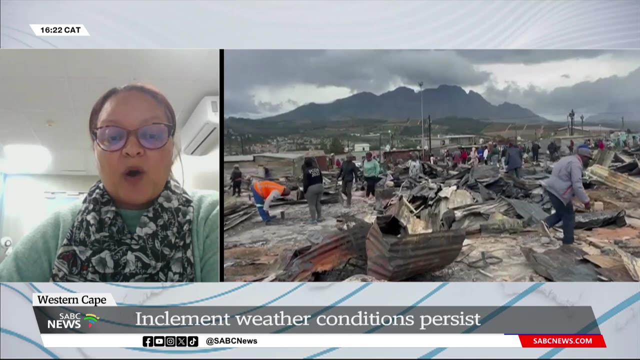 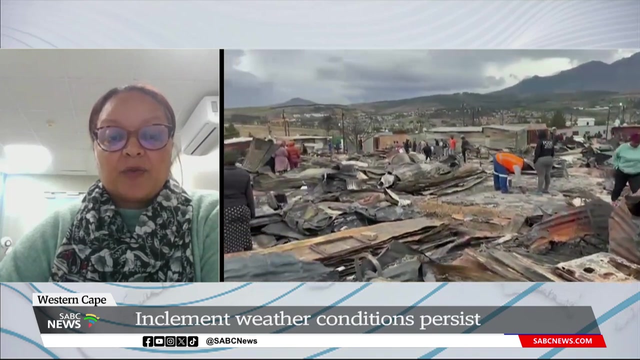 of land in Monwa and 247 structures have been damaged. That's a true story. If there's any leaks of any sort, don't feel socient. yet There needs to be changes that have been made, because over the past couple of 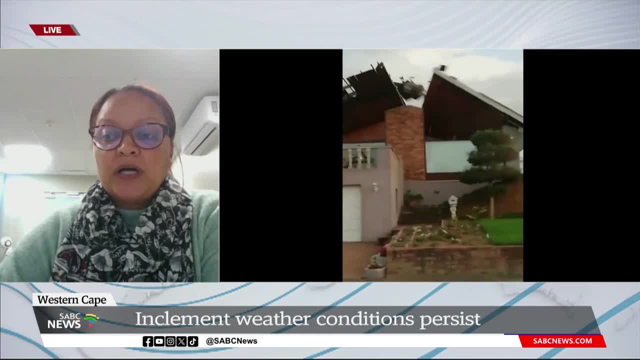 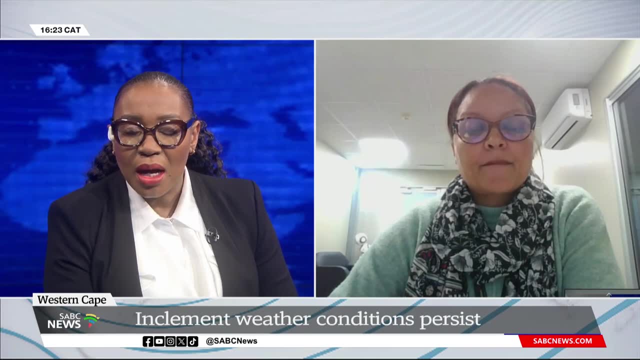 years, three to four hundred structures had been damaged as a result of flooding. opini underst 나왔, busy to restore these areas And as we've heard, you know, from Gift of the Givers, you know, pleading, in fact, that residents should at least be, you know, evacuated. 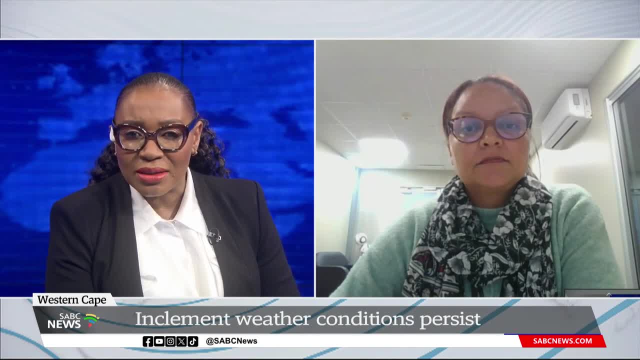 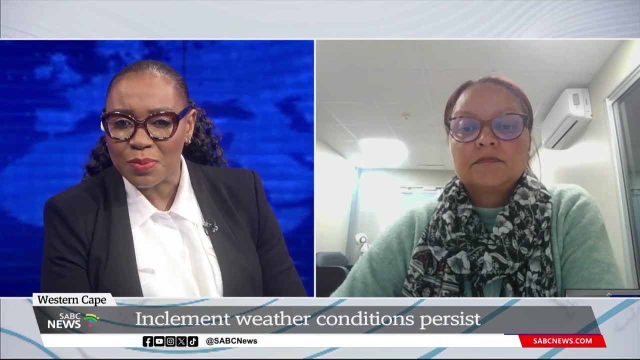 particularly given the fact that we are hearing that there is more persistent rain on the cards today. What are you doing in terms of alerting people, especially those that are vulnerable at this stage? you know to move to shelters, I would imagine. 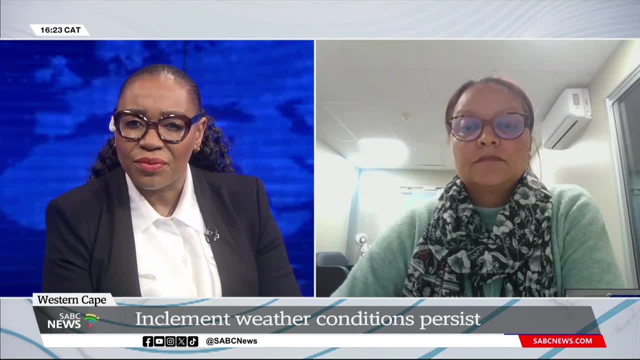 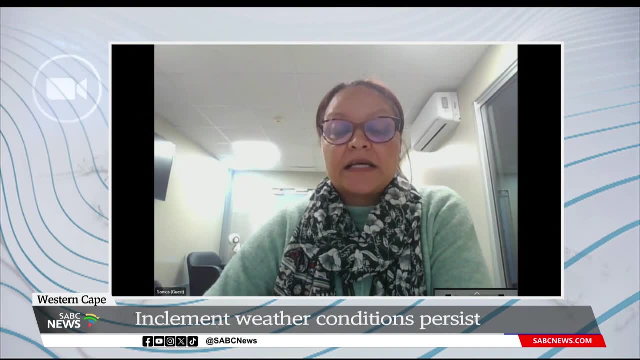 Just talk to us about those arrangements. Our disaster management risk officials are on the ground busy monitoring the high-risk areas and also do some awareness in the areas in terms of moving to taking up shelter at friends and family. And then we also have our RIMS department. 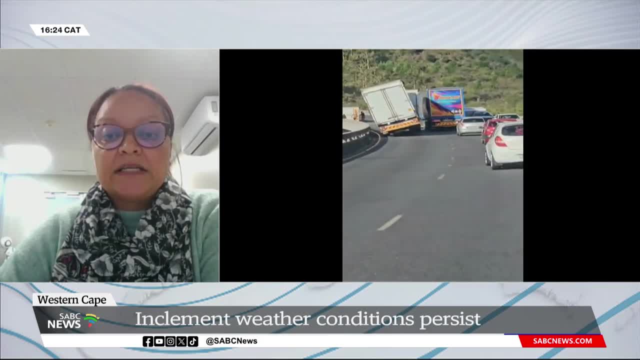 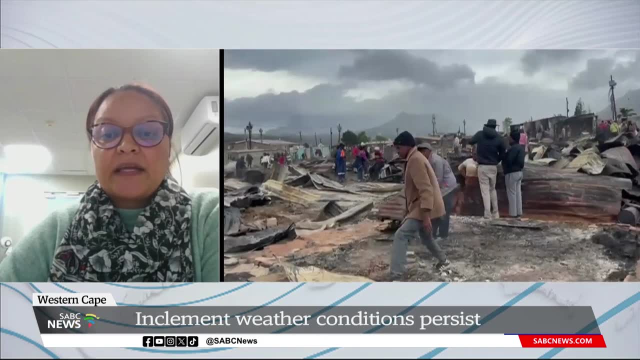 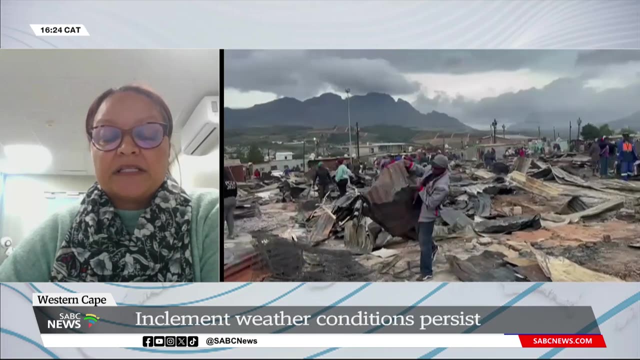 who is assisting with sandbags in some of the areas where it is needed, And we are also our informal settlement areas also busy. We are also busy seeing where they can assist with flood kits. We are basically engaging with our National Human Settlements Department in this regard. 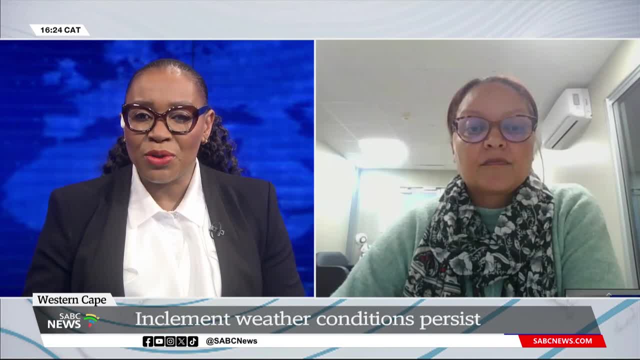 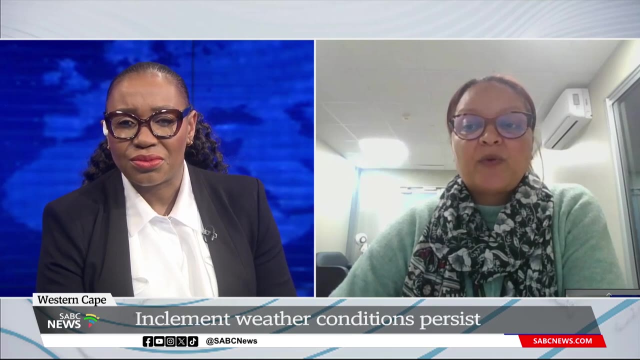 So we understand, of course, like I said earlier on, you know one person was killed. we understand today in Pal. Just talk to us about any other incidents, any other injuries. Is everyone? how is everyone doing In the city of Cape Town? we haven't received any reports.